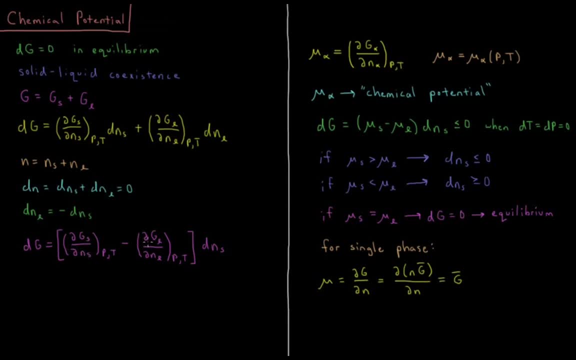 with respect to number of particles, minus the partial derivative of the Gibbs energy of the liquid with respect to number of particles, Each of those being at constant pressure and constant temperature. So now, with these derivatives popping up in this equation, it's convenient to define a new quantity. 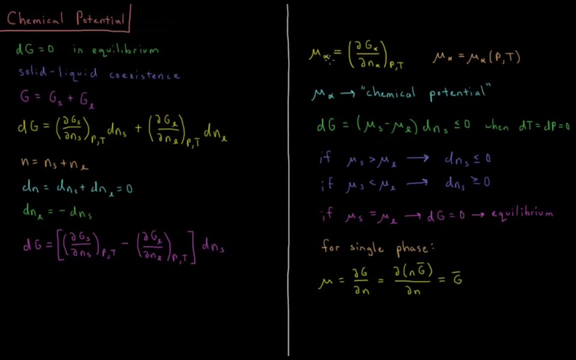 We're going to say mu alpha is the part of alpha being a phase. So mu alpha equals the partial derivative of the Gibbs energy of phase alpha with respect to the number of moles of particles in that phase at constant pressure and temperature. So mu is a function of pressure and temperature. 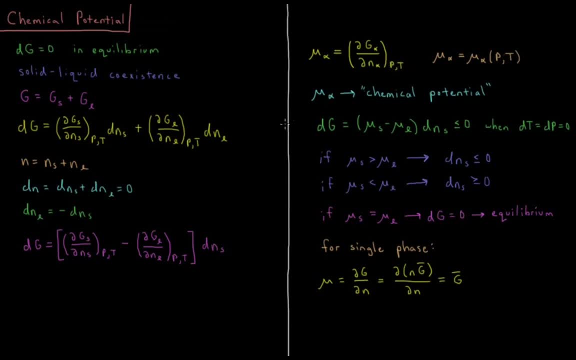 as we can see, because we're keeping both of those constant there. And mu alpha is called the chemical potential. So it's the change in Gibbs energy per number of moles of particle in that phase. So the change in the Gibbs energy from changing the number of solid and liquid particles. 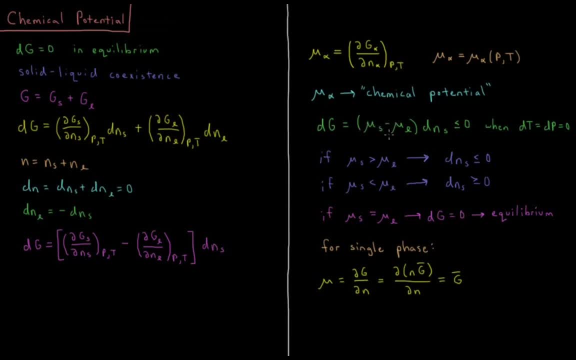 is the chemical potential of the solid minus the chemical potential of the solid times, the change in the number of solid particles And for any spontaneous process in a closed system at constant temperature and pressure, this quantity has to be less than or equal to zero. 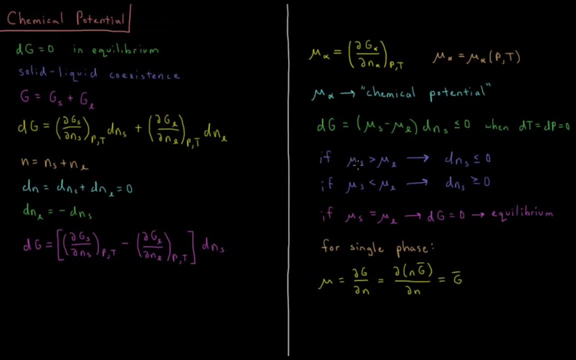 Alright. so what if the chemical potential of the solid is greater than the chemical potential of the liquid? So if this is greater than this, that means this is greater than this. This quantity is greater than zero. So for this whole quantity to be less than zero. 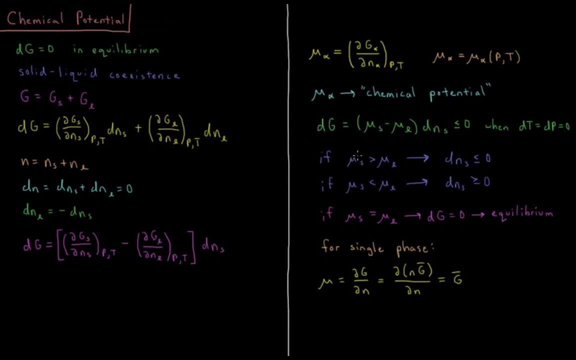 dns must be negative. So if the chemical potential of the solid is greater than the change in the number of solid particles must be negative. Particles are flowing from high potential solid to low potential liquid. If the reverse is true, if the chemical potential of the solid is lower, 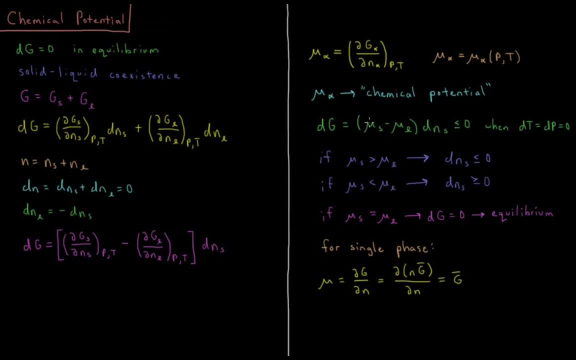 than the chemical potential of the liquid, then this minus this is a negative. So for this whole quantity to be less than zero, dns has to be positive. So if the solid has the lower chemical potential, particles flow from the liquid to the solid.